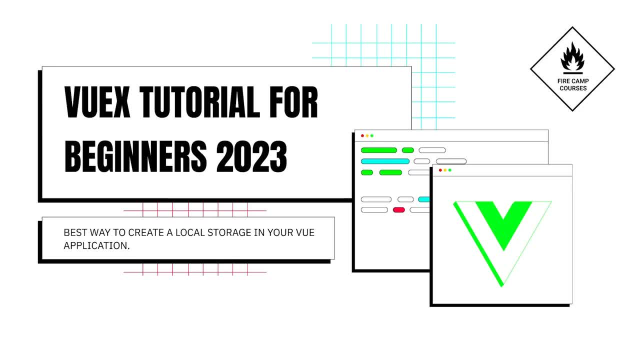 Welcome to Vuex tutorial for beginners. My name is Demyniko Stelny and today I'm going to show you how you can use this library in your Vuex project. So let's begin. What is Vuex? The first question 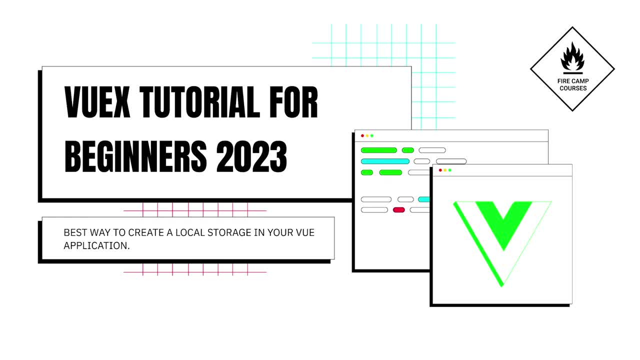 for everybody who heard about this library and knows that is used in Vuex apps is what is it? In short words we can describe Vuex as a local storage inside Vuex application where you can save some temporary data for example username, email or some tag, tokens or hashes. More about 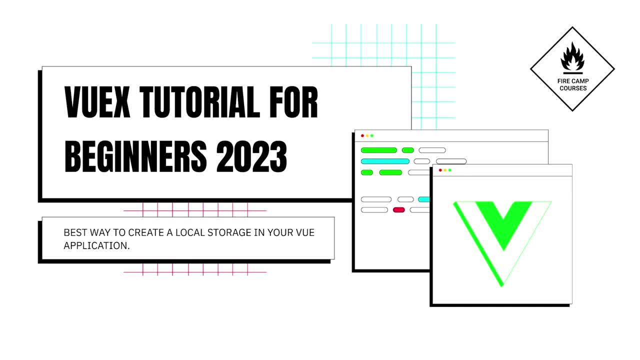 this you will see in this tutorial. So now let's go to the installation. Now we know what this Vuex is and that means that it's time to create a new Vuex application that will use Vuex storage inside. So let's do this. First let's generate a new application by its next command in our terminal. 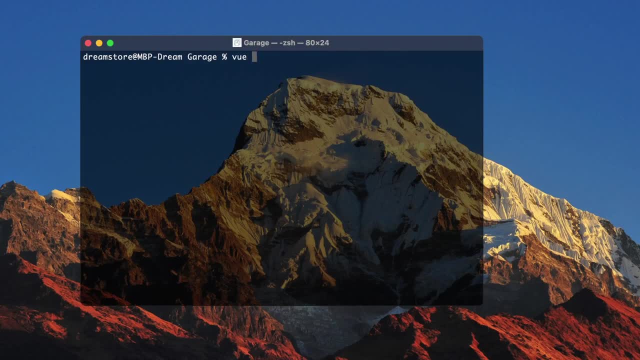 Okay so let me generate a new application as I said. So let's tap Vue create and for example Vuex example. So it will be the name of my folder with new Laravel or I mean Vuex application. So now let's choose Vue3. 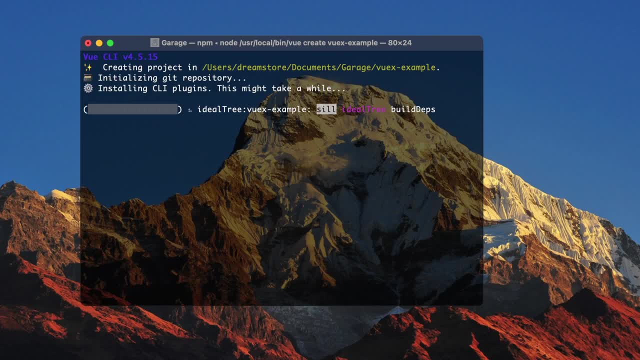 Vue3 version. And now let's wait until everything will be installed and after that we will go up to the project folder and install Vuex library. So let's wait until installation will be finished. 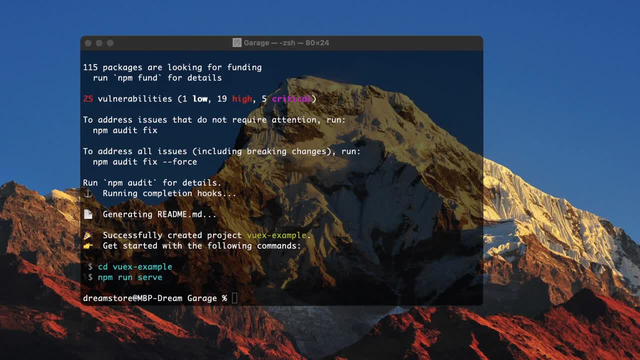 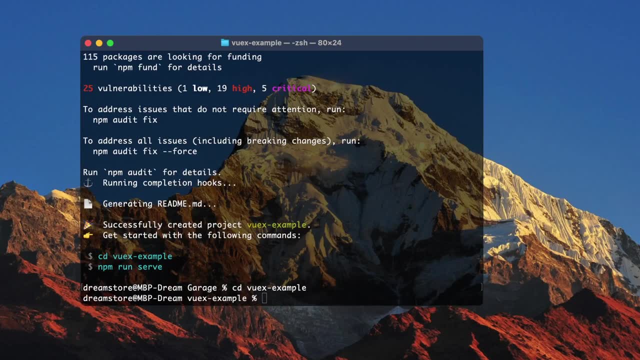 Okay so as you can see our app has successfully generated. So that means that now we can go to the Vuex example folder and now let's install Vuex. So let me show you npm commands that 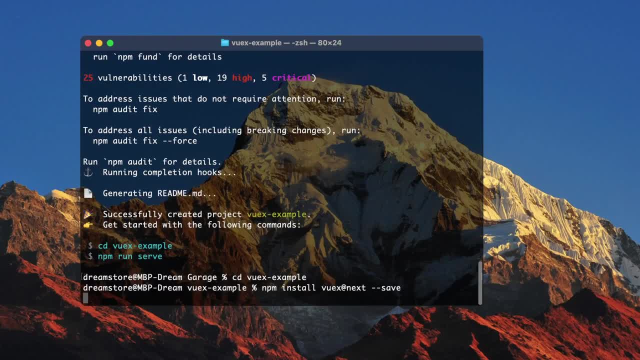 you will use to do that. So you will need to type npm install vuex-next-save and it will show us the vux. Go to the vux app webpage and just type vux-next-save and git open. 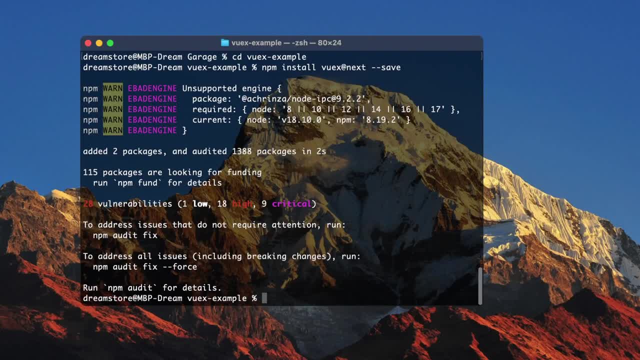 It will show the vux app with the vux-next-save command. So you will need to type vux-next-save and it will install Vuex library so as you can see everything's fine yeah also we can use here npm audit fix 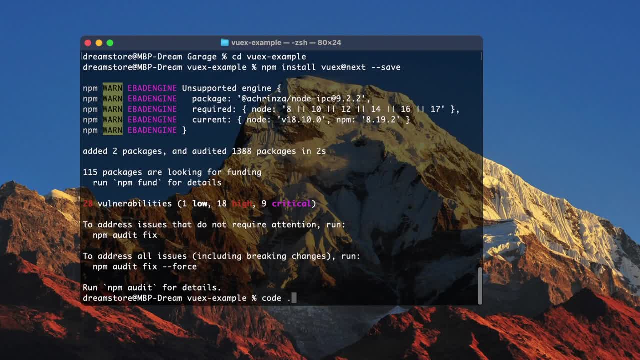 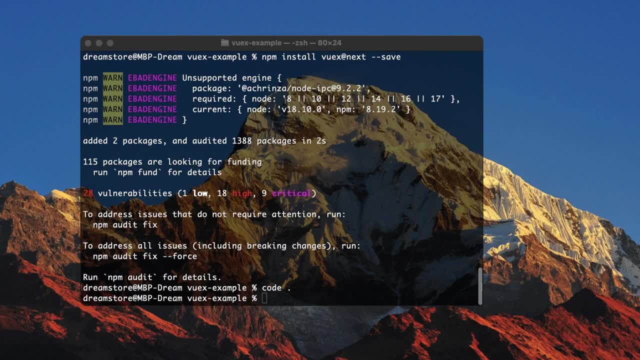 force for our packages but now I'm going to open my project that I just generated in visual studio code so let's do this okay and now let's see what we have and what we will do now so let me show you 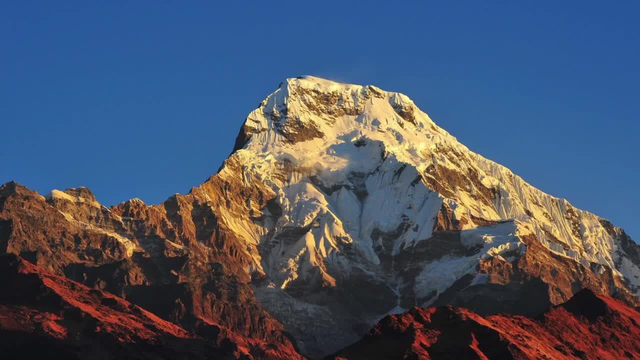 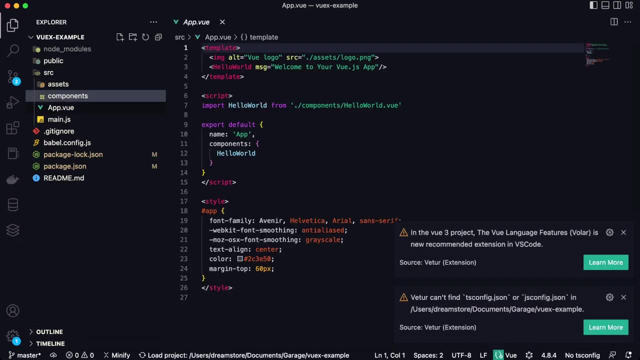 my visual studio code that I opened at my project okay so I'm here and as you can see we have default by default created app.vue component and hello world also so first let's you know let's 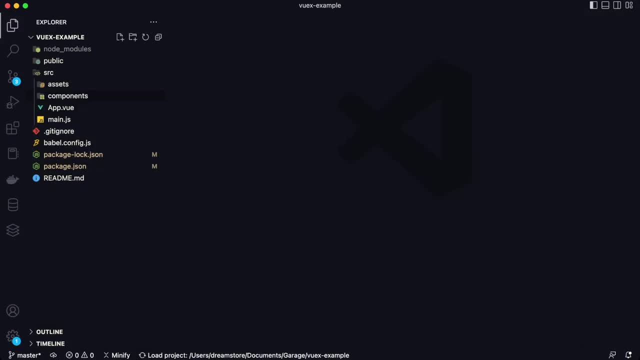 delete this component hello world and yeah let's also remove this component from the app.vue yeah also in this tutorial I'm going to use composition api so before we're gonna do some 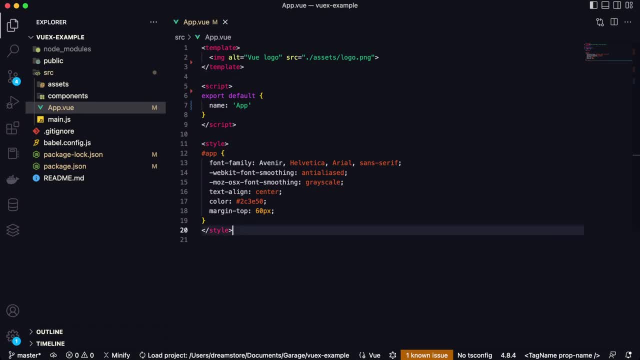 examples with this let's clear all this stuff so let's also delete this sync and let's type here for example ux e 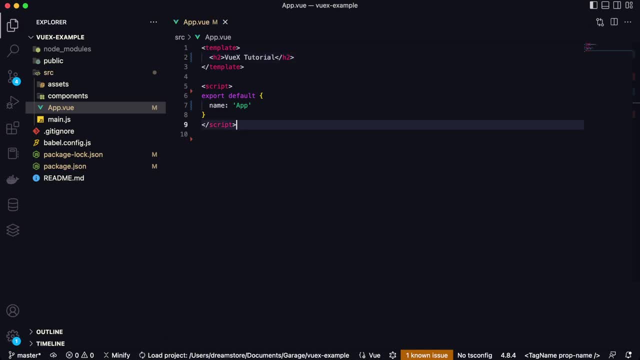 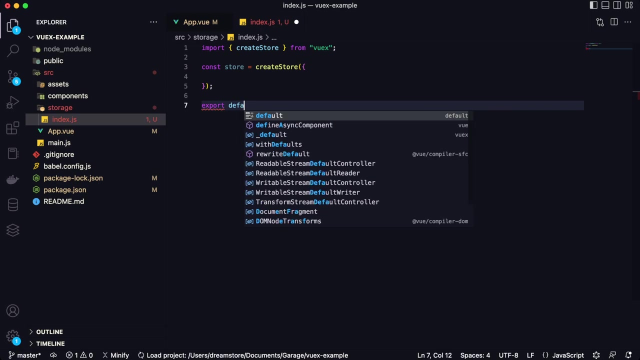 tutorial okay so now the first another question that we have hope we can set up vx in our project so to do that you will need to generate a new folder inside the src folder named storage and inside this folder you will need to create a new file named index.js so in this file we are going to type everything to that we need to create a new storage of our application and first let's import function named create store from ux so first you will need to import this function and after that we're going to create a storage so let's type here const store and after that we will need to call this function create store and after that we open here object where we're going to type parameters and also variables that we'll have in our storage after that let's type here export default store and let's type here state so the first question what state in short words we can describe this like a object where we can define all variables that our store will have so for example let's imagine that i want to have a new variable in my storage that will be saved and will be named count and by default this variable will have zero as value okay so that's the way how we can create a store first you type this function and after that you 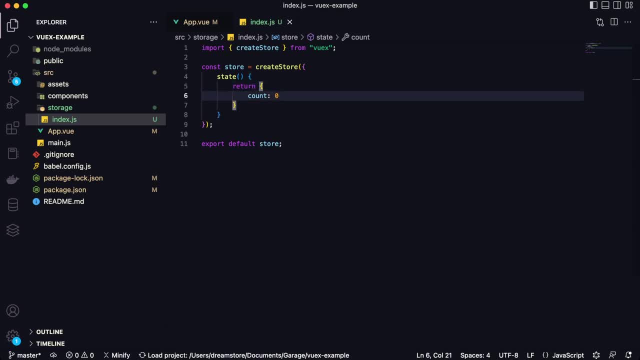 return here object that have every variable that you want to save in this store 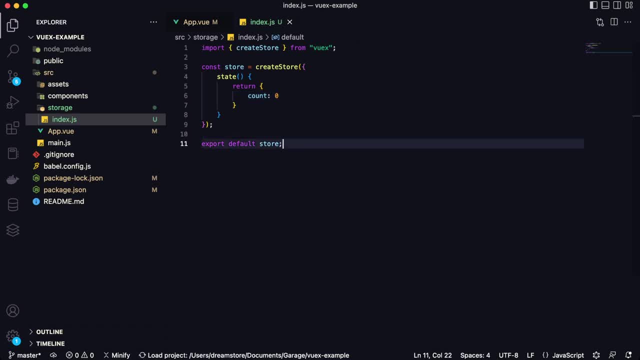 okay so yeah that's all for now that's all that you need to know now let's try to do one example 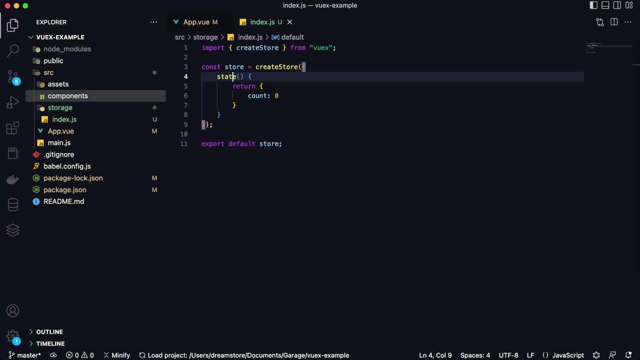 so the first concept of the view x this is state and and state as i said it's like a object where you define variables of your storage that you have in your view application so now let's create a new 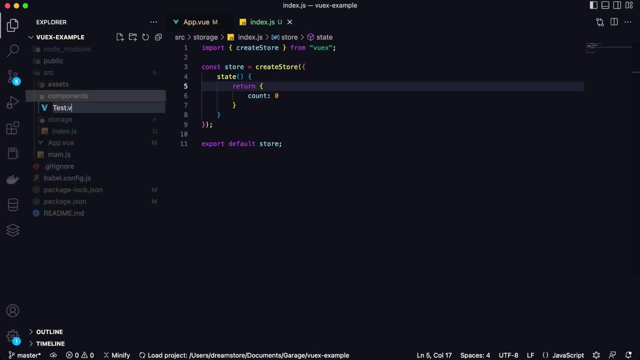 component here for example test.view okay and as i said in this tutorial tutorial i'm going to use composition in api so let's 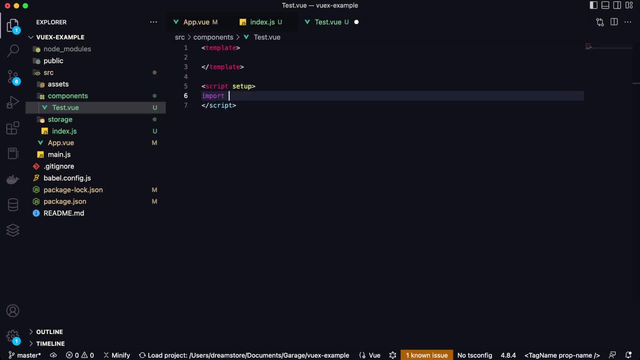 type here script setup and now we can import our store so one of the ways is type import store from from storage okay and for example let's imagine that now i want to see what i have in my storage so i'm going to type here store just yeah so just console.log my storage let's type here storage 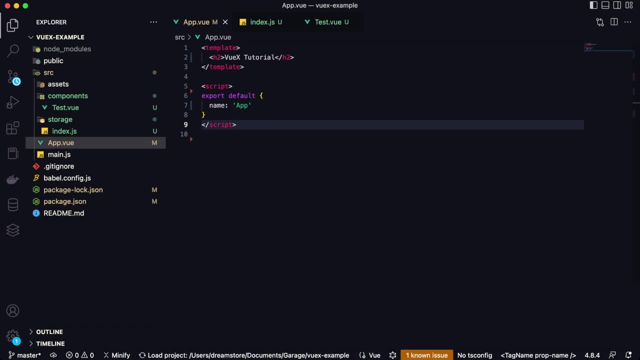 test okay now let's go to that view and now let's import our test component so let's type here import test from dot components test dot view and let's open here components object let's define it in this component we want to use test component and let's type here and show this 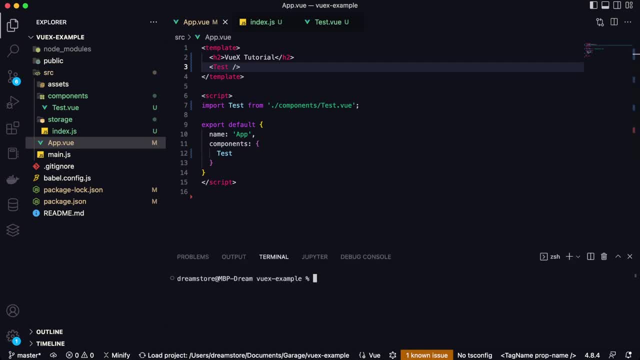 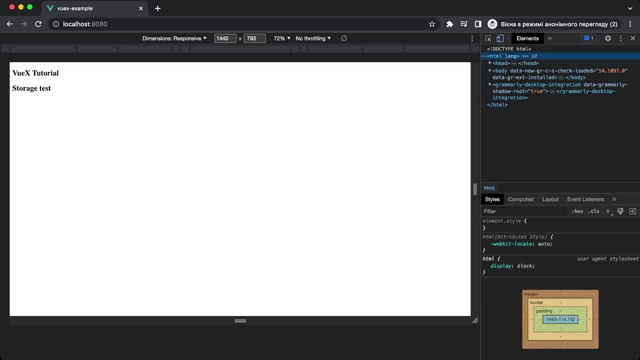 component so now let's open terminal and now let's run npm run serve okay so let's see as you can see server successfully started so now let's go to the google chrome and let's check how this works okay i'm in my browser and we can see here view x tutorial storage test and let's open me console 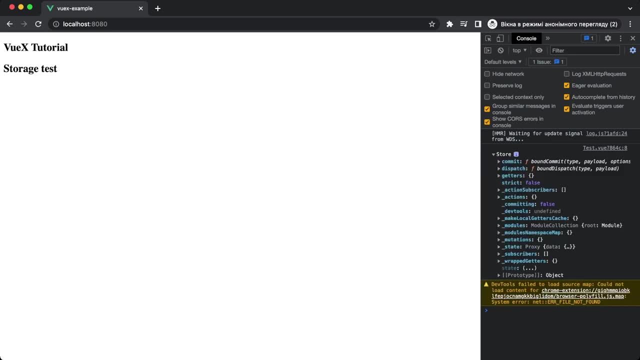 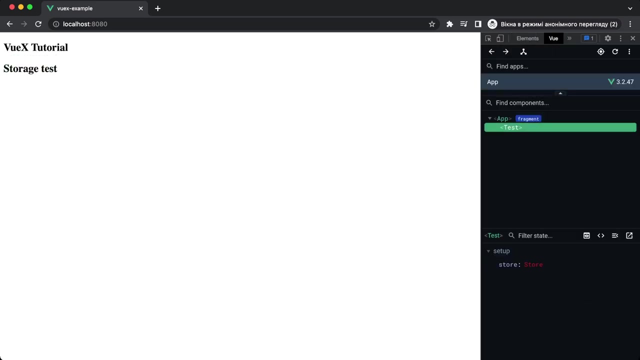 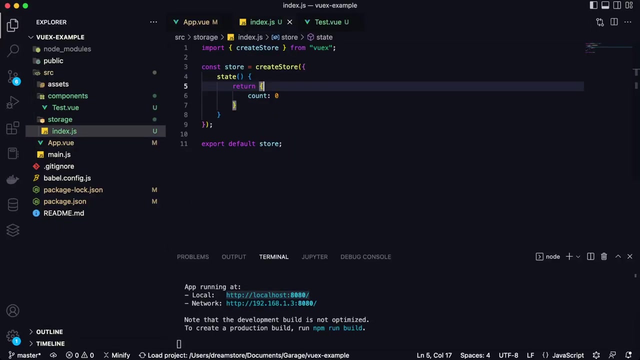 so as you can see we have store and we have some getter some other functions and as you can see here we have one variable name state and if you open this you can see we have data but we can't open data yeah no if you go to target you will see data and here you will see variables that we successfully created here so count but if you will use view plugin you can also open this and you can see that we have to test and as you can see here we have also store so as you can see view plugin see that we're using store in our view project and yeah that's all that we have in setup so that means that we successfully created storage in our application and you know now let's try to do one example so for example as i said we have this count variable and let's imagine that we want to increment this value of this variable and let's show this in our view project so let's go to our test data component so let's do this if you want to change value of the sum variables that you have in your storage in vx you will need to use features that is named mutations so somebody asked wow what is mutation we can describe mutations like uh you know like methods that we use to change value of the variables that we have in our state in our storage let's imagine that we will have here function that will be named increment oh yeah and also i forget one important thing yes i created storage but i forget to add this storage in my main.js file so 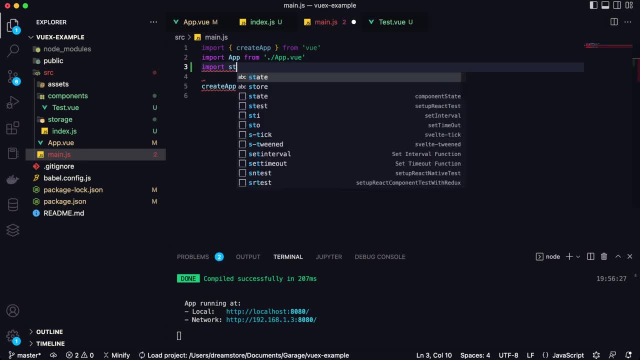 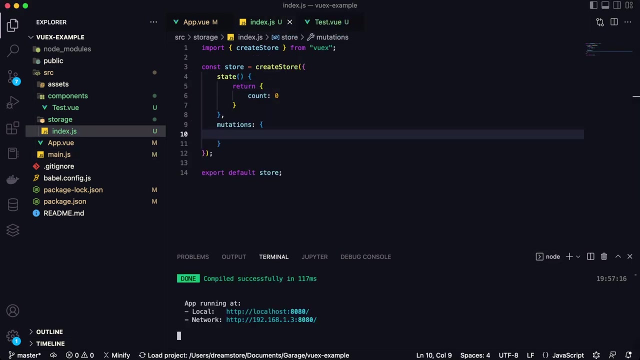 that's one of the important things that you will need to do so type here store from from from from storage and let's type here app.use store okay so now i fix it i forget to do this but this is really important to define that you want to use uh your store in globally in your component in your app okay so i fix it now let's get back to the main.js file so let's get back to the main.js file so let's get back to mutations so as i said we can define mutations like a custom functions that we can use to define to change value of the variables that we have in state or for example we can manipulate these data that we have in this variable so when you're creating a new function in mutations you will need to create here a local variable named state and somebody can ask why we need to create this variable the answer is simple because by using this variable you will able to access state that you have here so for example i can type state and as you can see now i can access to my count variables that i created and i can change value of this variable and if i save it and now i can call this mutation but somebody can ask questions so wow how we can how we can call this mutation uh so now let me show you how we can do this and but first let's create here a new variable named temple count and let's define that it will be maybe ref or maybe you can just type here store state count so yeah 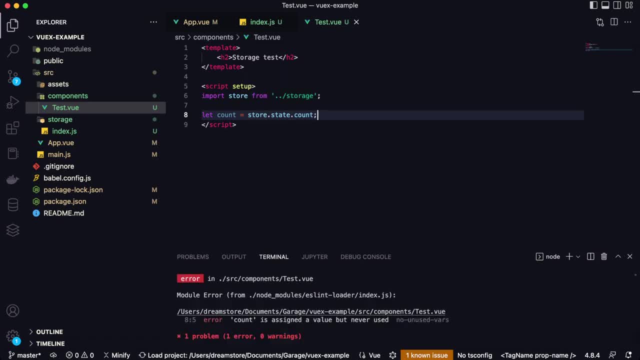 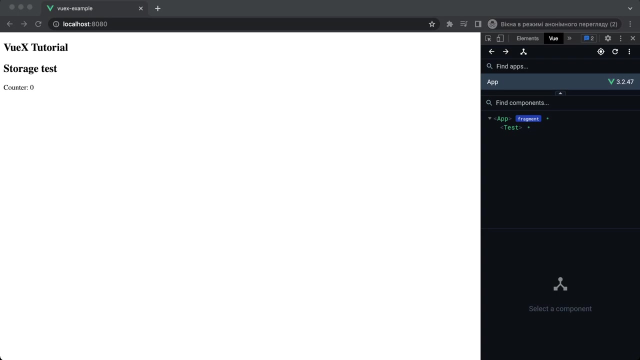 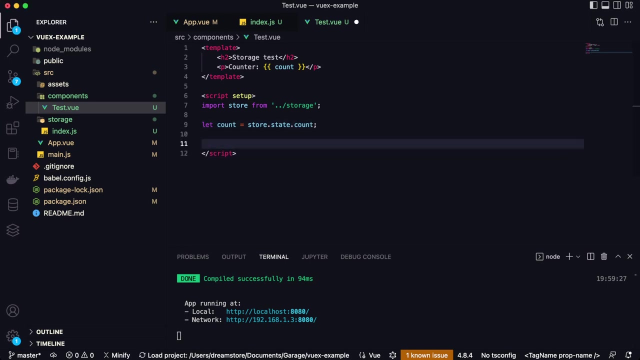 for example if you want to oh yes it will not work okay oh no yeah so this is working okay so if you want to use some variables that you created in your storage in your component you can just create a variable and after that define store state so you enter to state of your storage and after that name of the variables that you want to show so for example i'm going to type here counter and my count variable so as you can see now everything works and if i try to open browser i will see that i have counter that equals zero so if i go to test you will see that our count variable is equal to zero okay let's get back to results that you got and now let's make some changes to call here mutation that we just created so if i want to call mutations that i created first i'm going to create here a new function for example call increment and here i will type just store commit and name of my of mutations that i want to call here so for example commit increment and yeah so as you can see call increment is defined but never use it now let's use this function so for example uh let's create a new button named his name increment and let's add here click event so call increment and yep that's all that you need to do if you want to call mutation that you created in your storage also i'm gonna show you how you can provide some variables 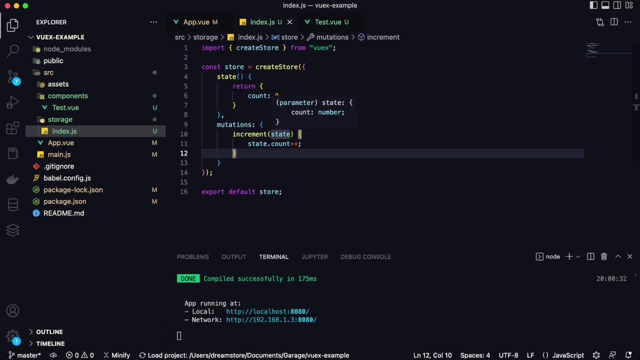 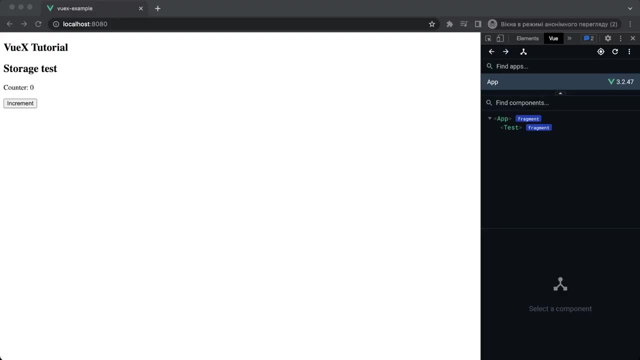 and values inside mutation because you can create other variables in your mutations that you created okay so now let's try to check it so let's get back to browser and we can refresh it and let's go here let's type test and let's click increment and as you can see we have one trouble with increment increment button so we'll 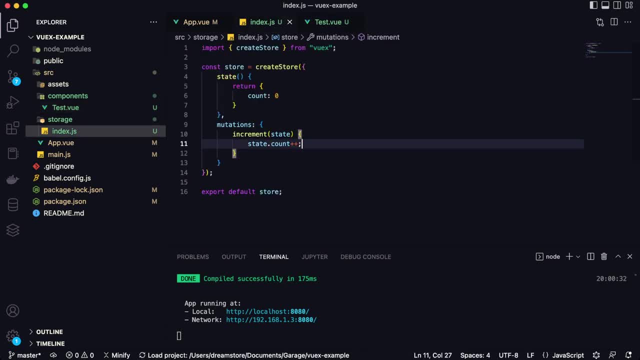 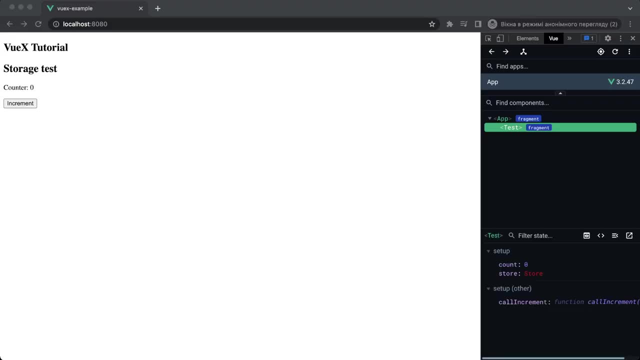 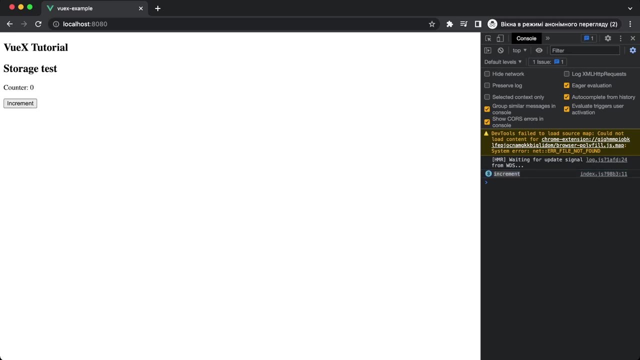 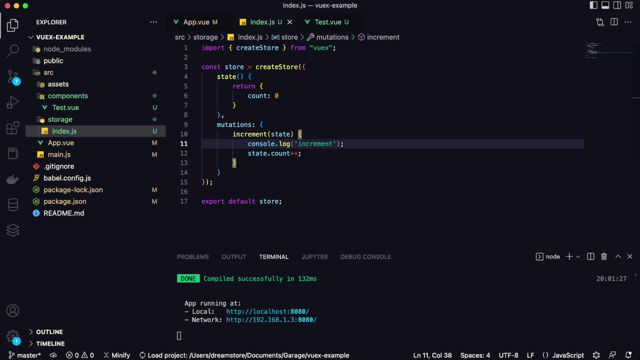 like i did something wrong here so maybe first let's first let's type here console.log increment let's see that our mutation is called okay so let's open here console and let's type increment and as you can see that mutations is successfully called but we don't change value of the state of the maybe of the state no i think not we changing we don't changing value of the count variables that we created here so let's try to do this by this way or we can just define this as ref as i 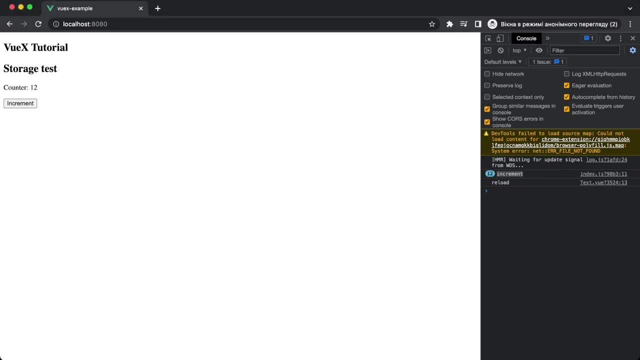 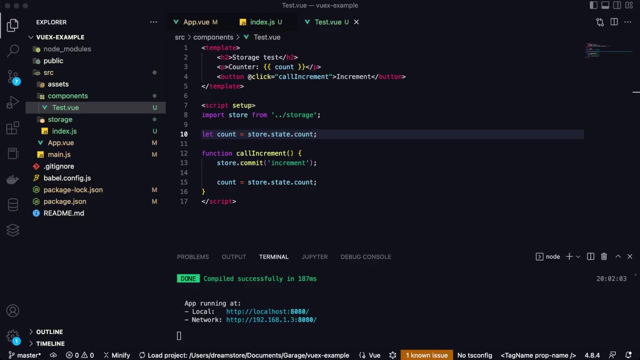 said but let's try first slides this way and if i now as you can see pages refresh it and if i click again if i refresh as you can see value is not changing so the problem is i think because we don't use in here ref so let's get back here so we can define here ref and it's because i'm using 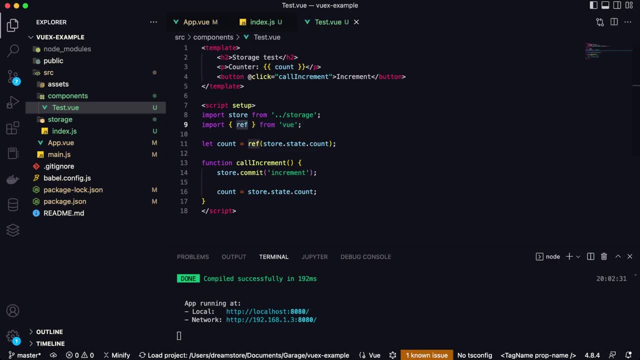 composition api i will need to also improve my configuration here also so we'll just load it here so you can see and uh before we show here ref from view pack okay so let's open browser again let's type increment 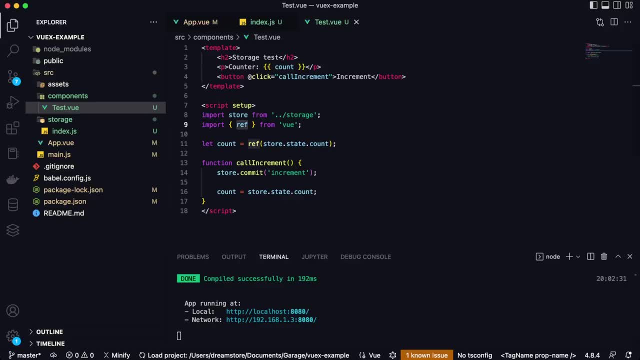 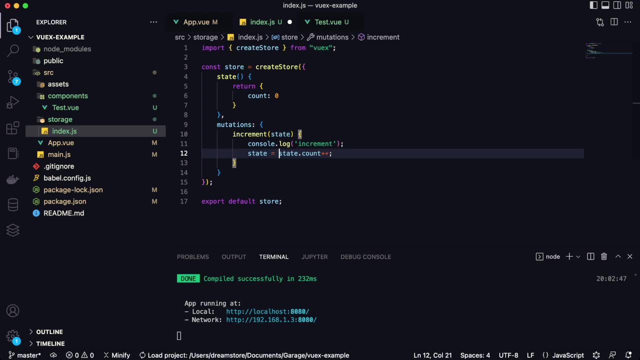 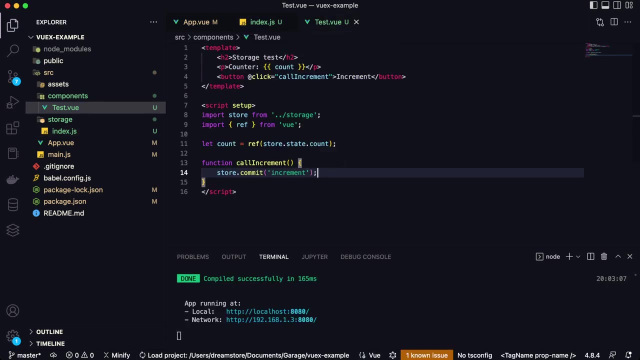 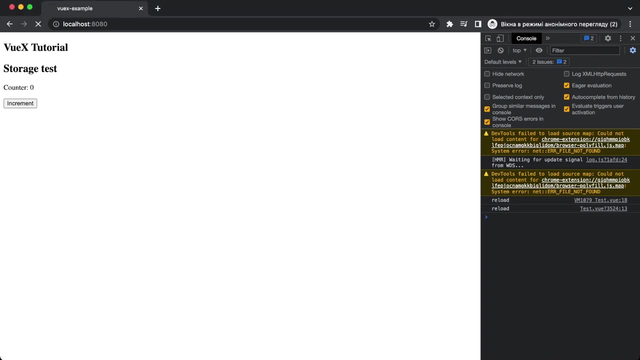 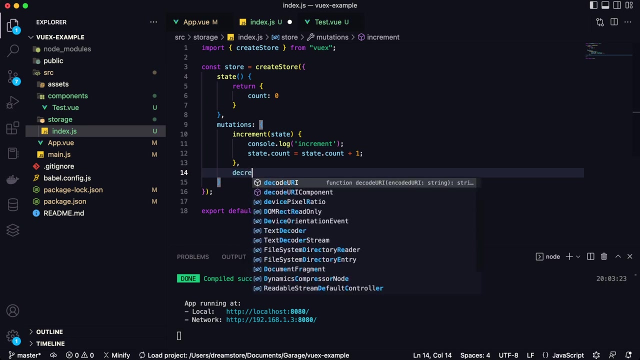 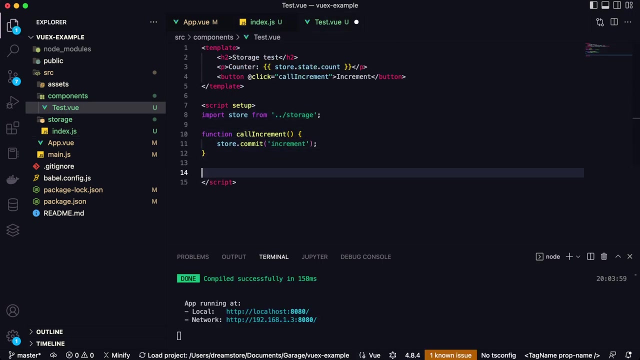 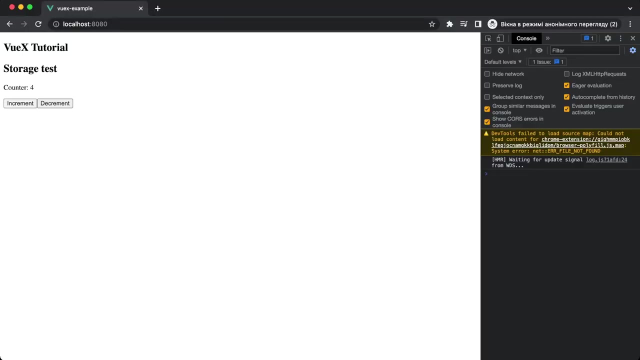 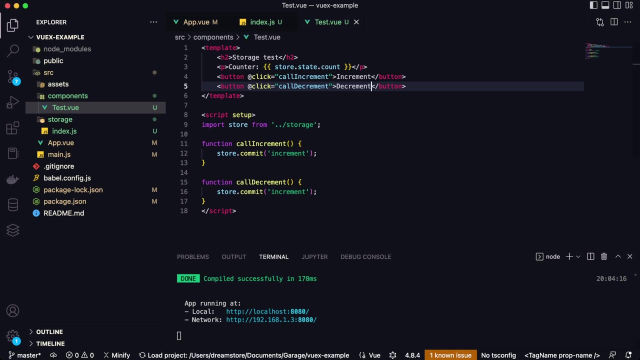 and as you can see this not work okay so maybe I think we have some trouble with state changing so maybe we can just try to type here state count equals count plus one or something like this and we can go here again but you know maybe we can just type here store count store state that count and ref is defined by the user so let's change this and okay everything is fine here so let's get again the browser let's refresh it and now as you can see everything's work so it was trouble only with variables that they created and as you can see our mutation is working so that's great for example we can now create another mutation that will name decrement so for example let's type here decrement state and I can just type here so maybe we can first let's plus plus operators here and here here let's type here minus minus okay let's save it and let's create here call decrement function and let's copy this button and inside this button we're going to call decrement function and let's type here decrement let's save it and let's open browser again refresh it let's start try to increment and decrement and okay looks like i forget to change click event or maybe oh i 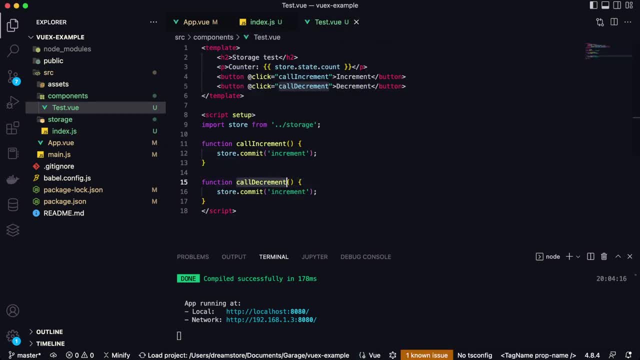 understand okay so i forget to type here name of decrement meditation that i want to call here 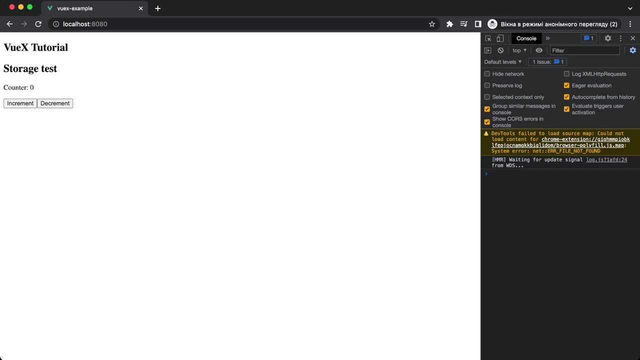 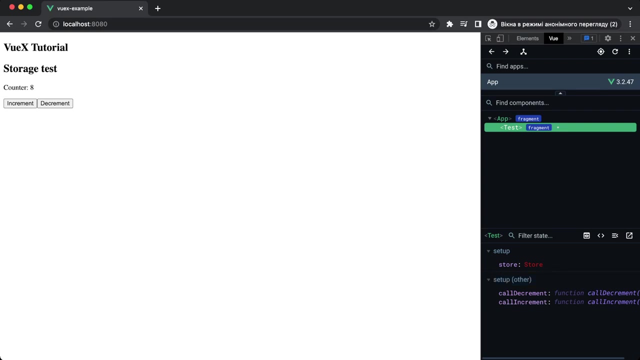 decrement meditation now let's get again to browser let's try to increment and let's try to increment so as you can see everything is store everything is now stored in local storage that we created here and as you can see we have call decrement function and decrement function yeah and increment function so everything's works and yeah so for example if you want to save some data 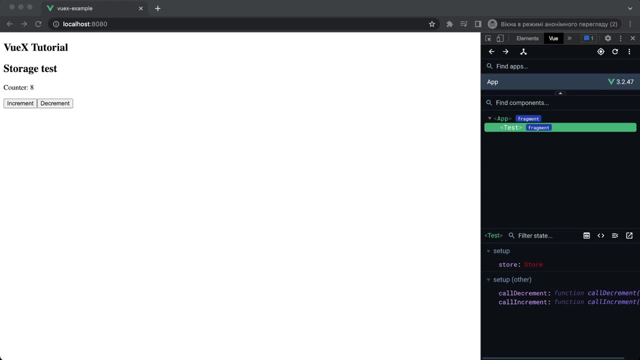 you want to change values of the variables that you created in your state of your storage you will need to use 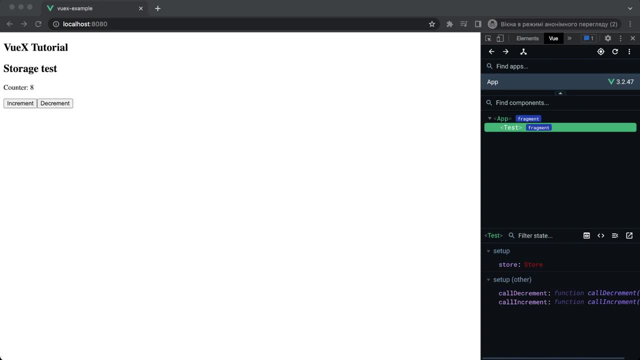 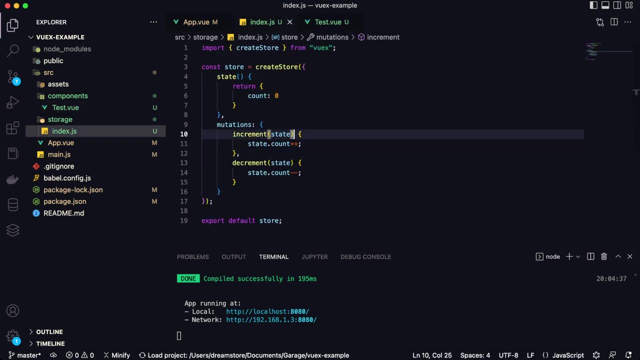 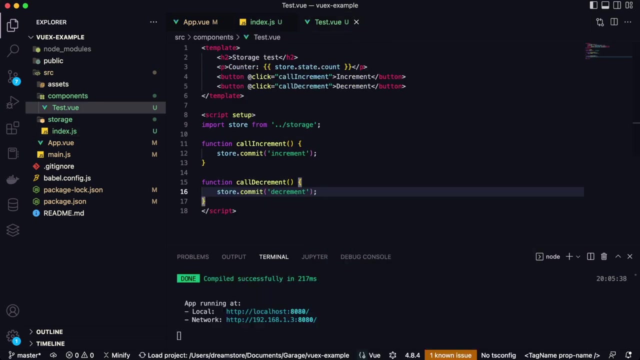 mutations yeah and now let's try you know another example so as i said you can create another variable in your mutation so for example let's type here and no number and let's provide this variable now in test.view so for example let's go here as you can see yep so i typed that so i 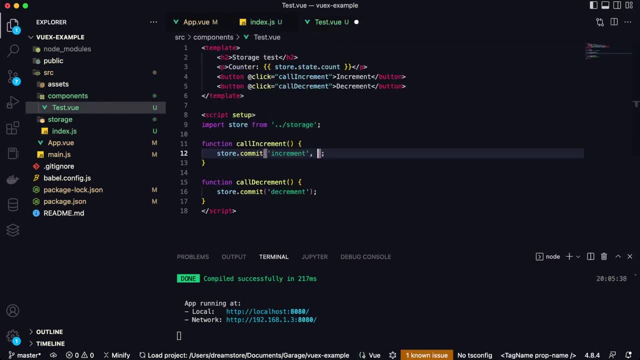 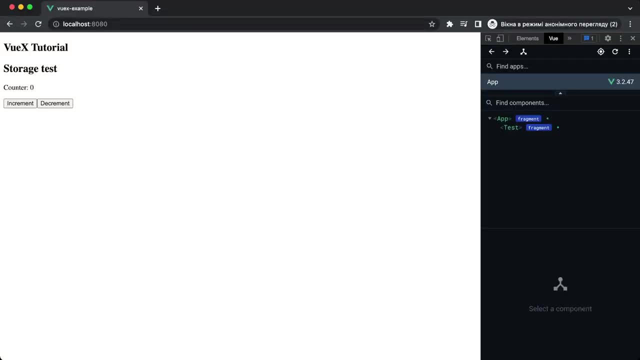 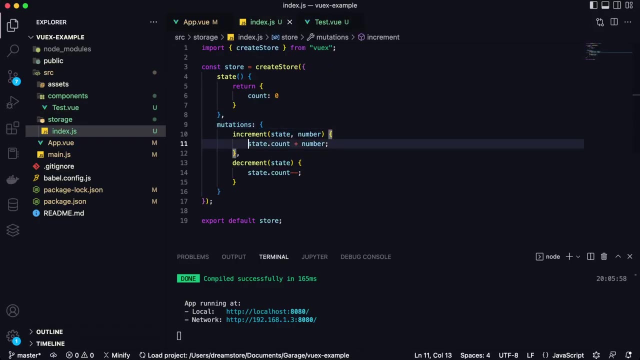 created here new variable named number and now i need to define the value of this variables that i just created so for example 50 let's save it and now let's open it and if i type increment okay so we have some trouble again okay okay so maybe um can type state count that counts equals this operation and let's type here number so we will see everything in console so increment 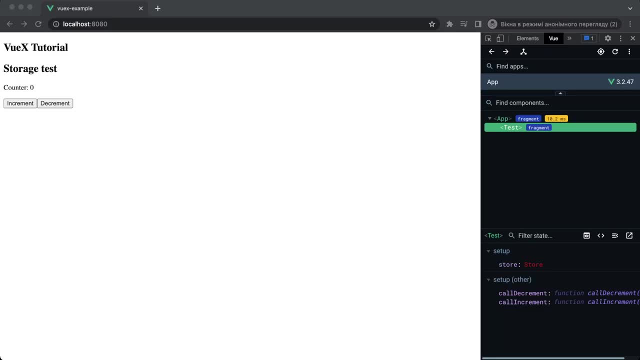 commit so now everything's everything must work so let's refresh it let's open console and let's try 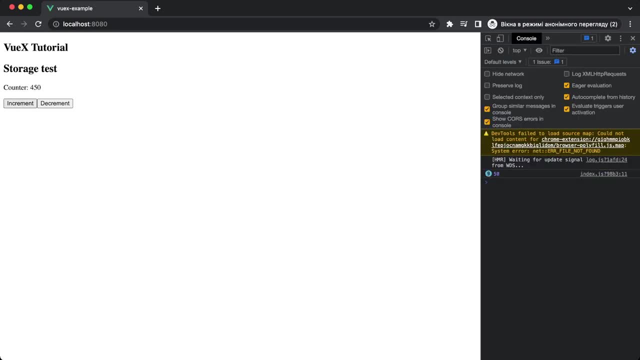 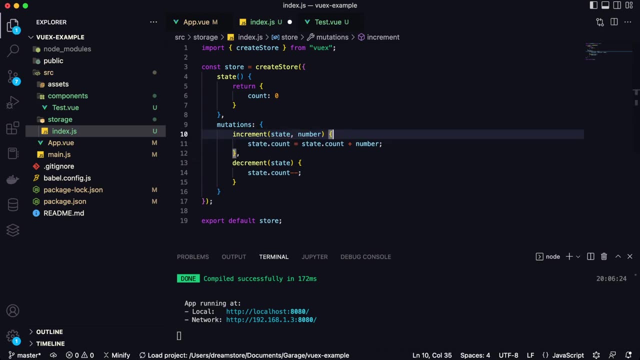 to increment and as you can see now everything's successfully working so the problem was because in my storage uh in increment function mutation i mean i forget to type that i want to change whether the 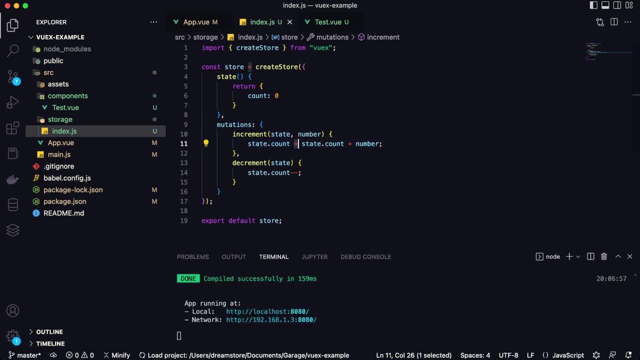 variable by this way and by using this operator that we use every time when we want to define the some variable so yeah so that's the way how you can type the way how you can create 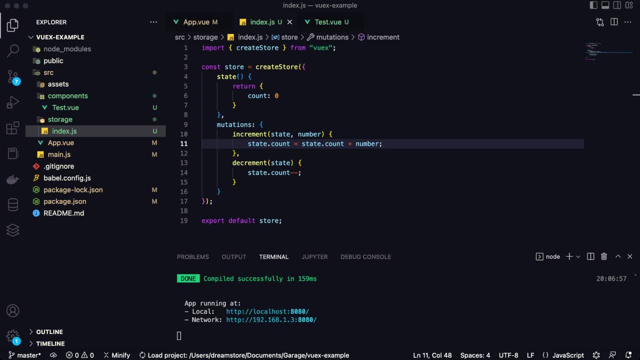 another variable variables in your mutation now let's move on to another concept of the 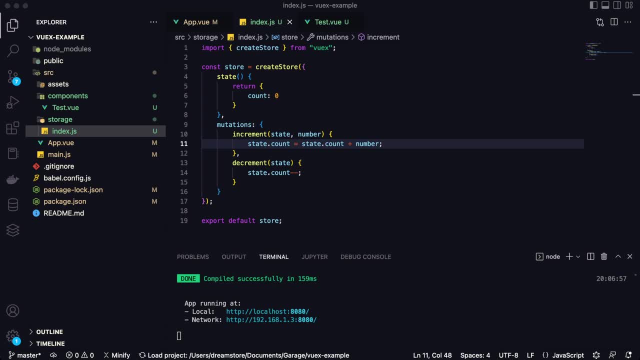 views and this that will be getters and actions so first let's talk about actions how we can describe actions so let's imagine that here i have action subjects and how we can use this 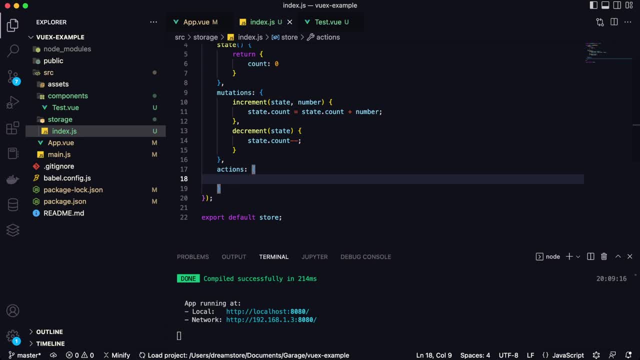 so we can define actions like functions which we can call and inside these functions we can call mutations so for example if you have operation um sets for or maybe a function where you want to 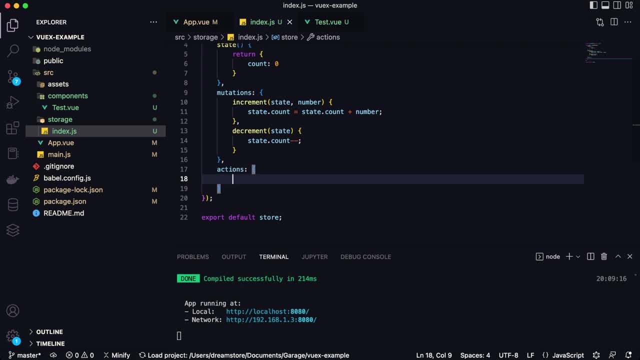 call three or five mutations and you don't want to you know create a function that will type every time commit commit comment you can just use actions so for example you can type one action 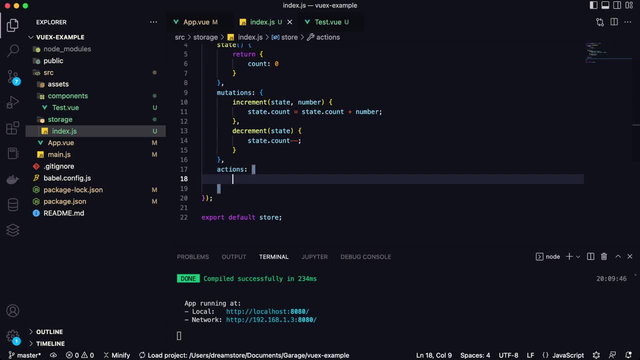 that will call for example three mutations so now let's start the function and let's see what happens let's create a new action that will make increment and decrement. So this action will call first 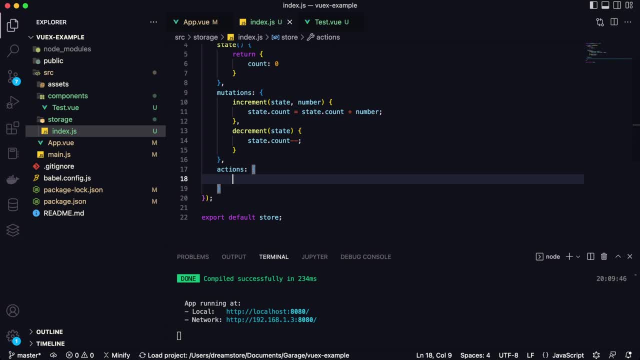 increment and after that decrement. So how we can do this? First let's create here new function 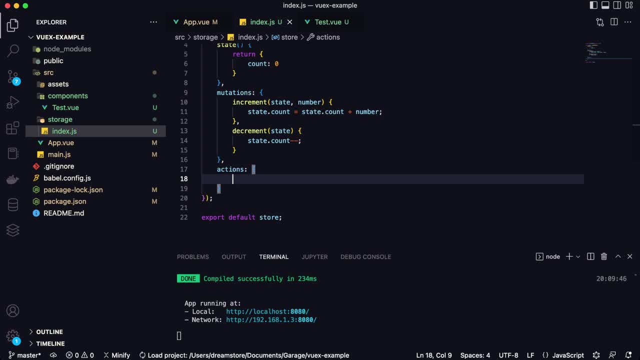 for example or maybe better to call this action that will be named like mega increment like this and here we will need to create a local variable that will be named context and by using context we can commit this mutation that we created here. So for example I can type here 50 as I did this 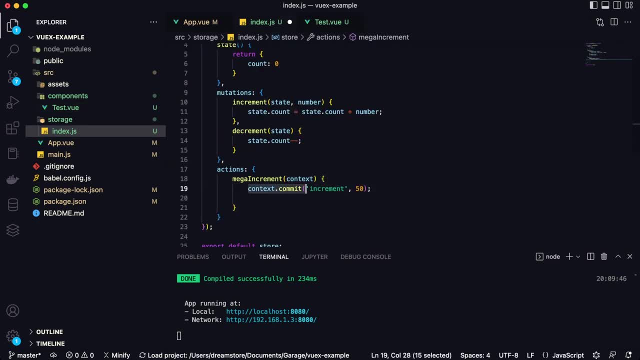 in test.view and here I can also commit second mutation decrement. So first it will add 50 to my count and minus one when we will call decrement mutation. Okay so now question how we 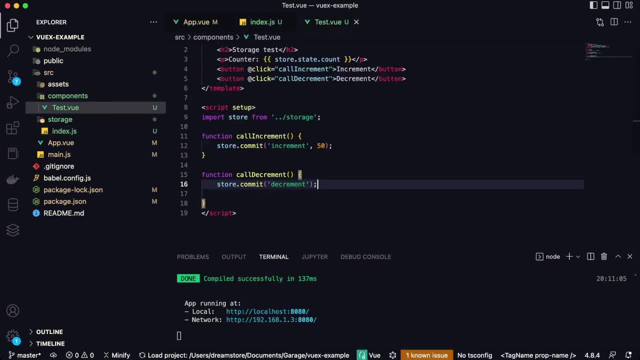 can call actions. So as I said you can use actions if you want to. So let's create a new action that will make increment and after that decrement. 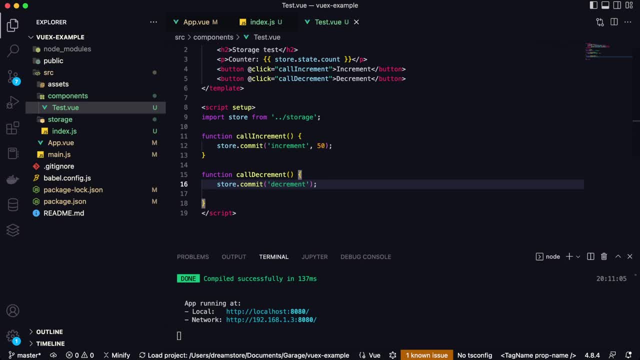 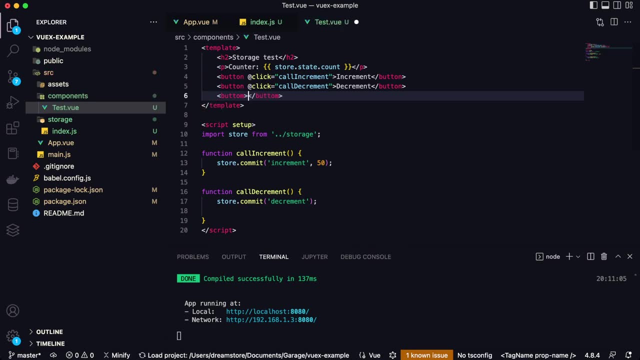 want to call you know three or four mutations or do some operations inside the app. So first let's create here a new button where we're going to type mega increment and after that let's define that we 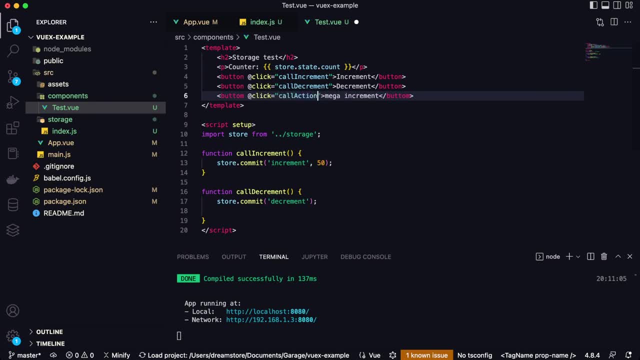 want to call here function call action and now let's create this call action function 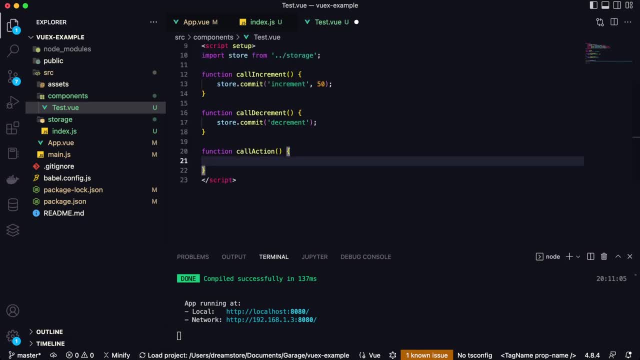 and let me show you how you can use and call actions. So if you want to use action you will need to click the action button and you will need to click the action button and you will need to 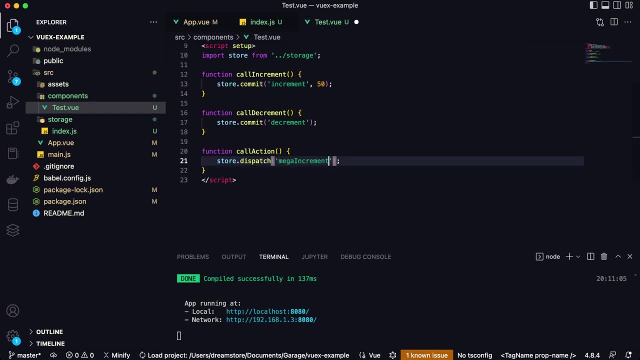 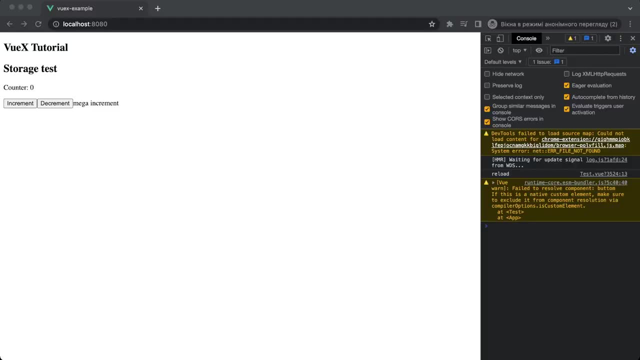 type here dispatch and you will need to define name of the actions that you want to call. So let's type here mega increment and as you can see everything is fine in console. Now we can open 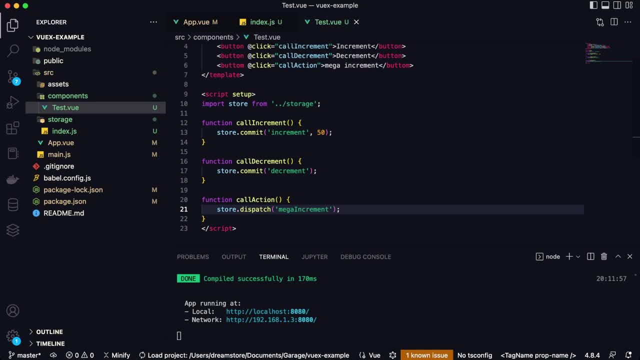 browser and looks like I did some okay I forgot to type here button. I type here bottom not button. 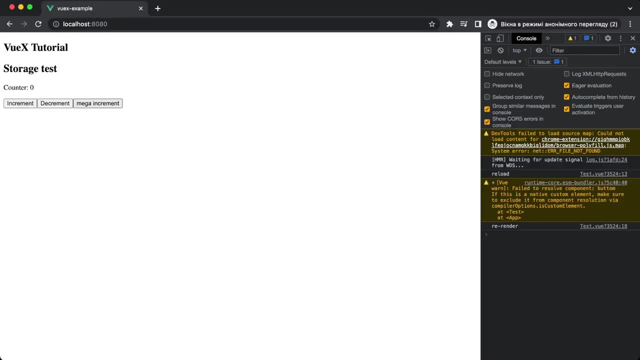 Let's refresh it and let's go to browser again and now let's type or I mean let's click on mega increment and as you can see first this calls increment functions because increment function is a function that can be used to count actions at 50 to count variable and after that we call decrement mutation to make minus one operation. So that's the way how you can use actions but you can 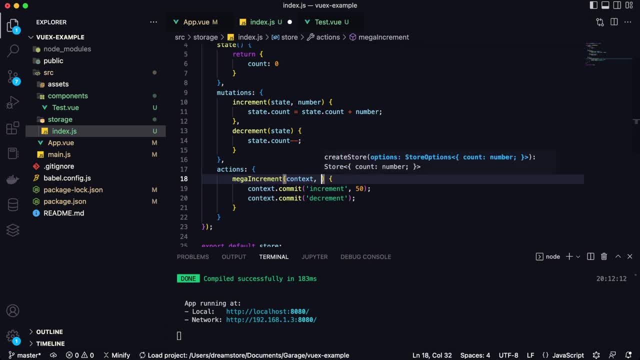 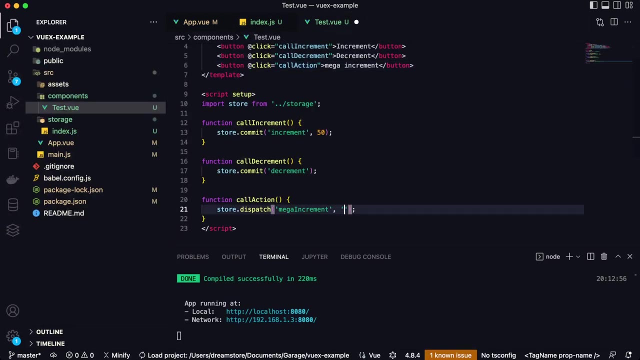 also create here variables inside action. So for example I can define here message yeah and let's type here alert message and let's go to test that view and let's define message that you want to provide here. So for example 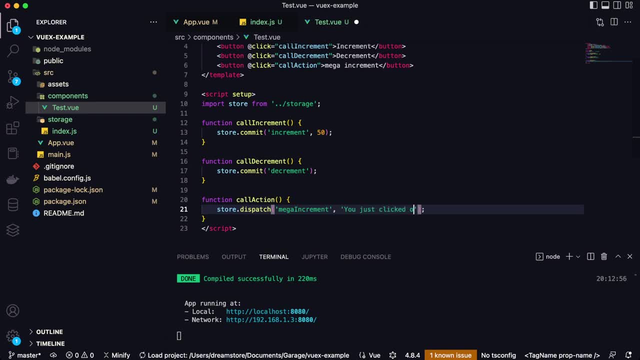 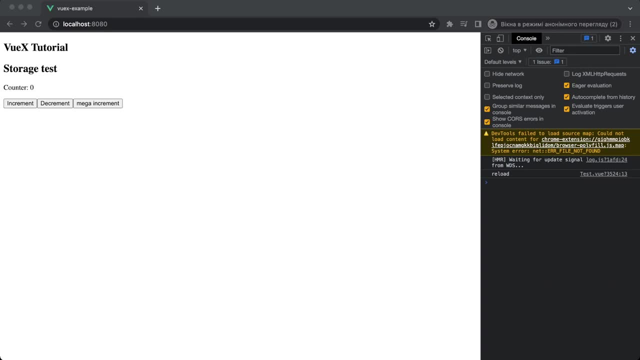 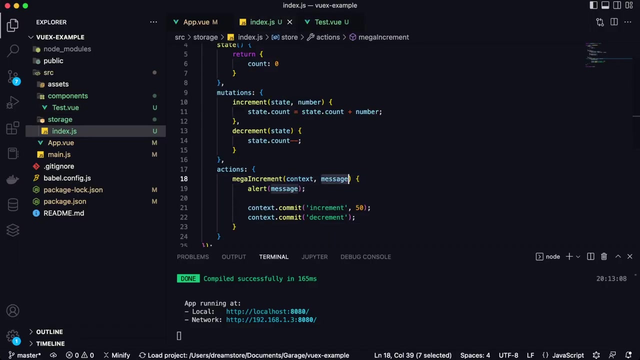 you just click it on mega increment button. Let's save it and let's go to browser again. Let's refresh it and if I click on the mega increment as you can see this calls you just click it on mega increment button and show this message and as you know we provided this message by creating here message 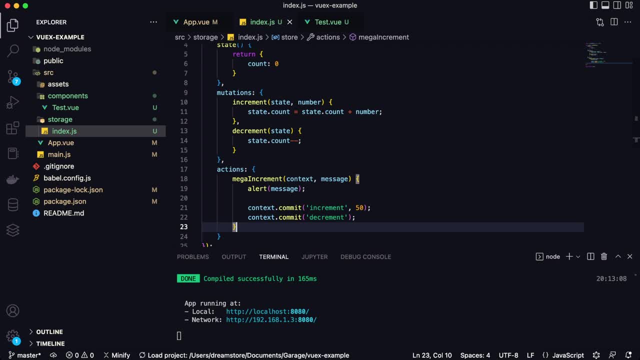 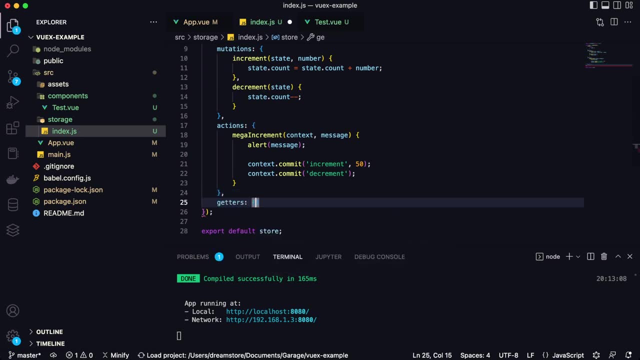 variable. So in actions you can also create here your own variables if you want in every action you can create here and now the last concept of the UX this is getters. So as name suggests you can 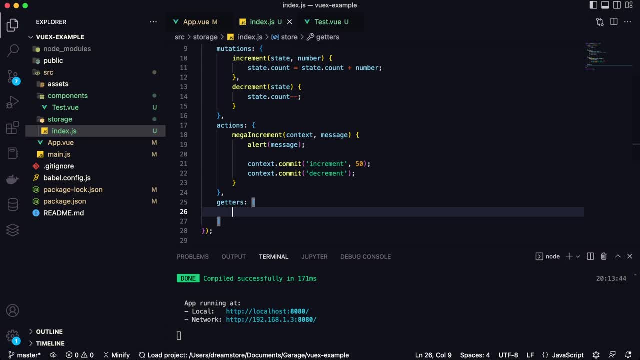 use this function if you want to get some data. So now let's do another example. So let's define that we want to for example return some data that will be multiplied by 10. So for example 10 multiply so it will be name of our getter and it will return state count 10 and yes state is not 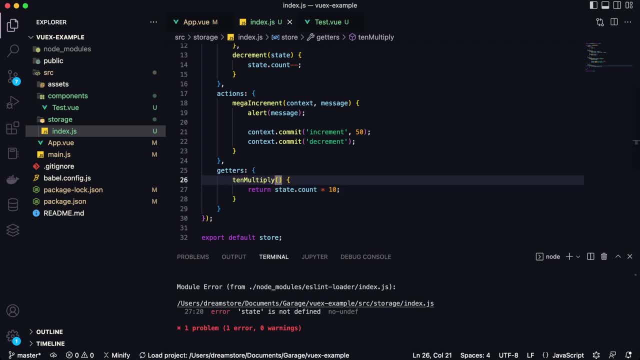 fine so let me fix it. So getters when you're creating a new getter you will also need to 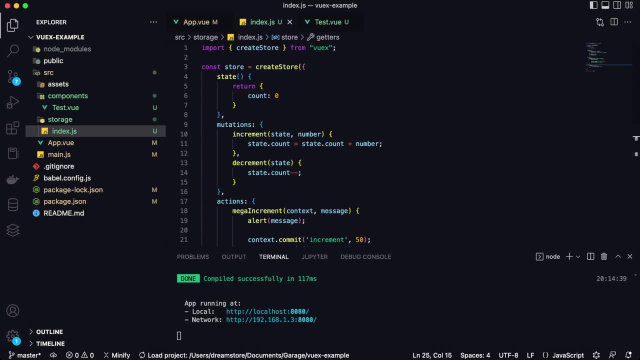 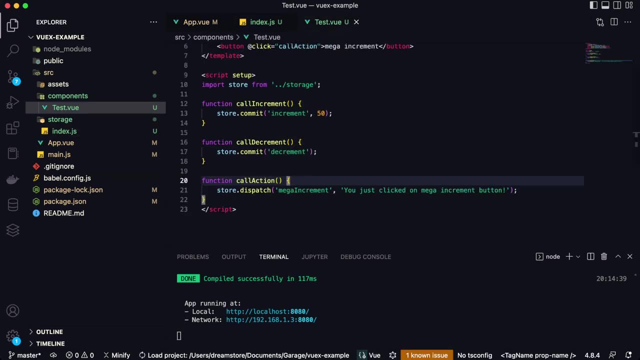 create here a state variable if you want to access your state of your storage and change values or get values of variables that you have in your. Now let's call this getter in our test.view component. 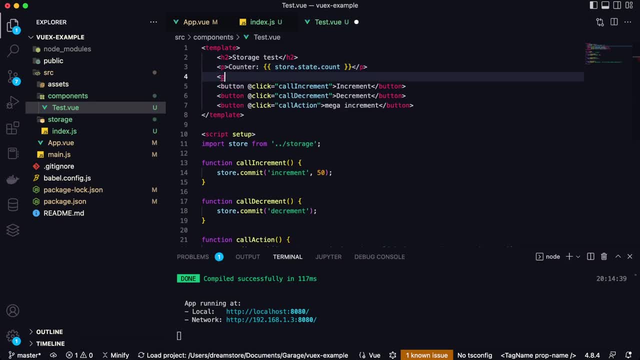 So if I want to get my getter and use it first let me type here using a getter and here I will type for getters and name of my getter so it will be 10 multiply. Let's save it as you can see we don't 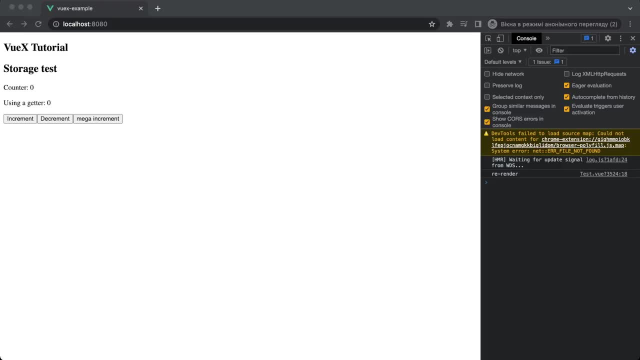 have any errors in terminal so that means that I can now open my browser and let's type here 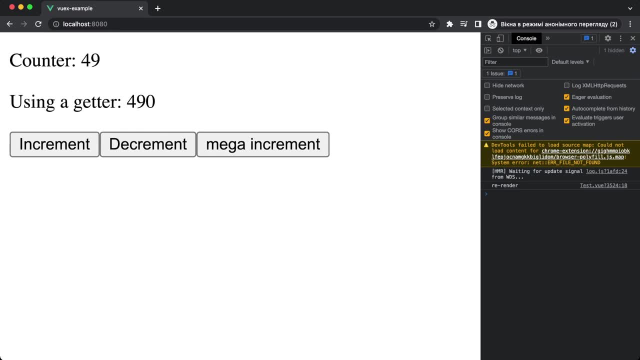 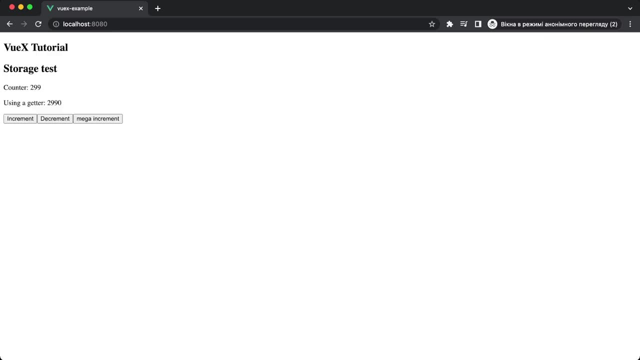 my increment and as you can see value that we have here is multiplied by 10 and I can type here increment and this multiplies. So that's the way how we can use getters. You can use getters 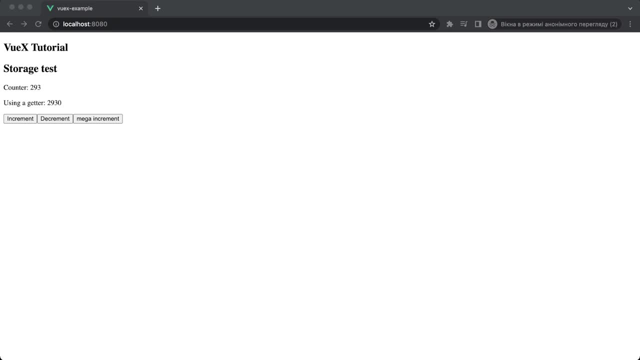 if you want to get some data and for example change you know for example let's imagine that by getters that you save some JSON data in your